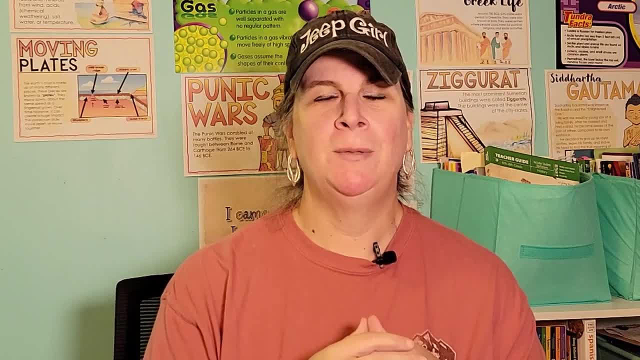 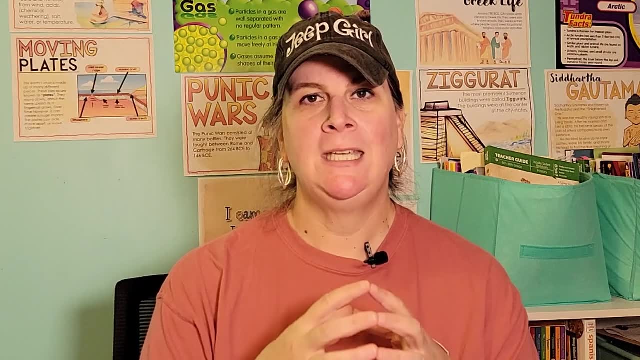 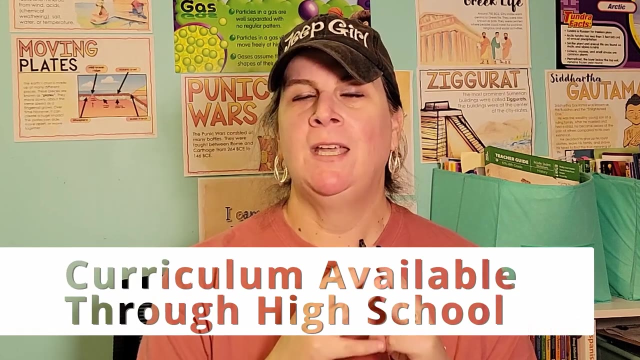 videos, although that was something that I was a little bit flexible on because I didn't know if I would be able to find exactly what I needed. But I wanted something that I could teach And then we could go to the videos when we needed to. number three: I wanted to find something that I would not. 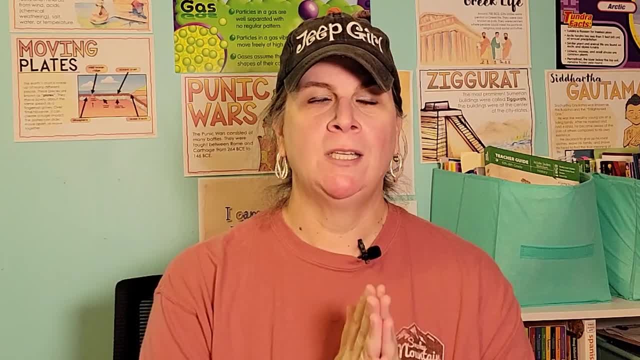 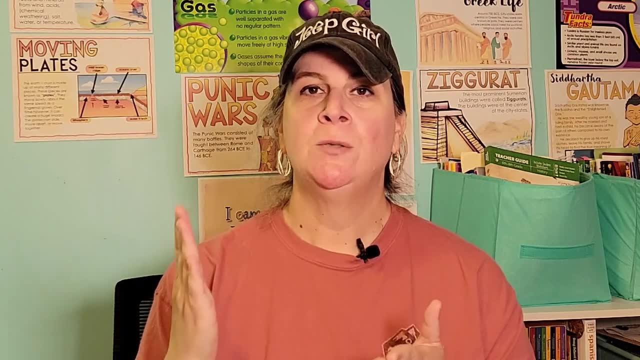 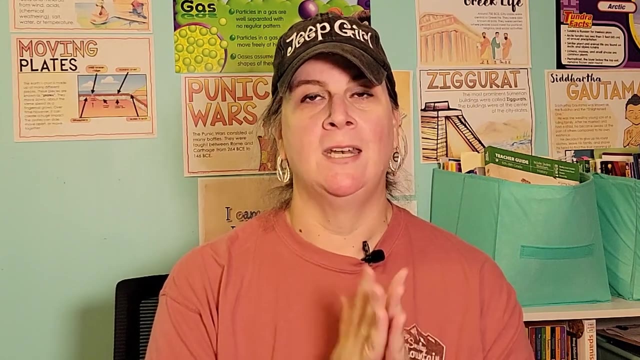 have to switch again. If this was a curriculum that worked for her, a format that worked for her, I, I wanted to be able to stick with it up through 12th grade, up through calculus, and I wanted to not have to worry about making this switch again. 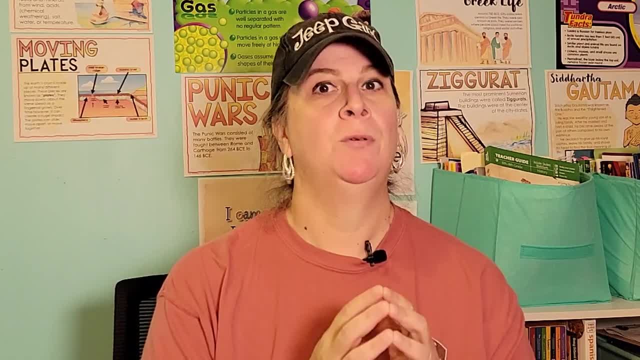 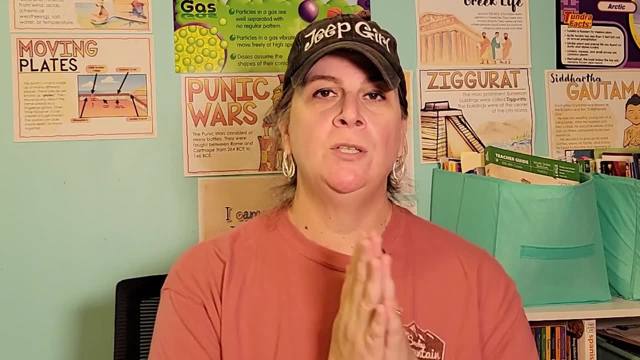 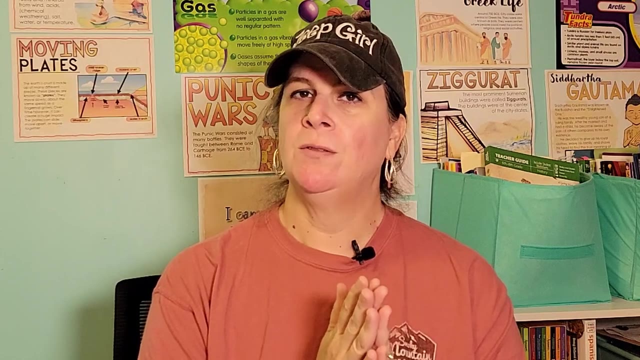 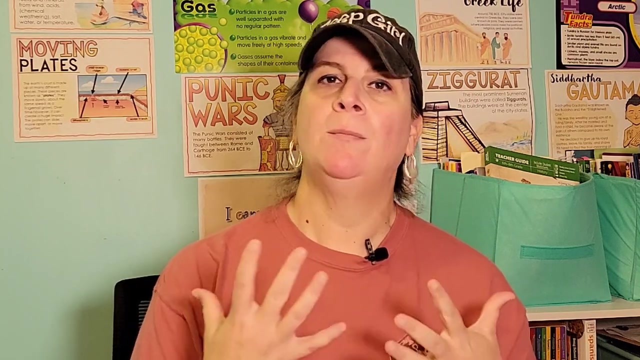 That was actually one of the most important deciding factors for me, because our switch from ABACA to Singapore Dimensions was definitely a very rocky one, And so I didn't want to have to go through that again, if I could at all avoid it. In today's video, I will walk you through what I discovered about some of the math curricula. 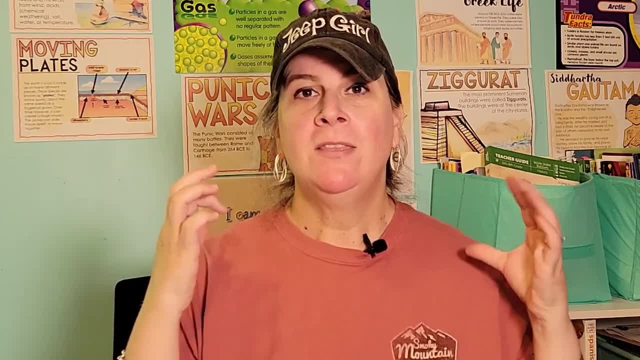 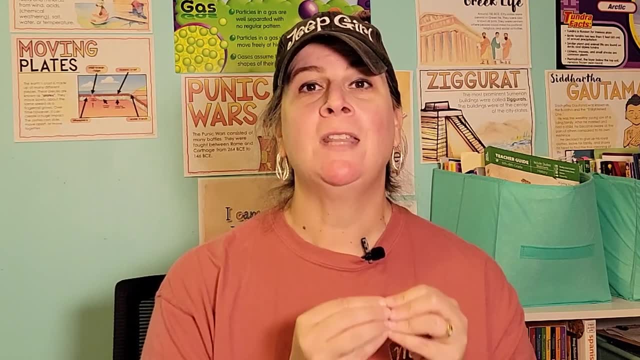 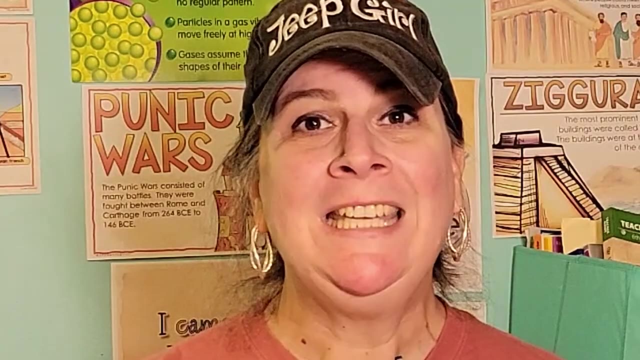 that I researched. This video is not all inclusive. There are so many curricula out there. I am very much a proponent of: if you find something that works for you, works for your student, your student is progressing and learning- then stick with what works, especially in 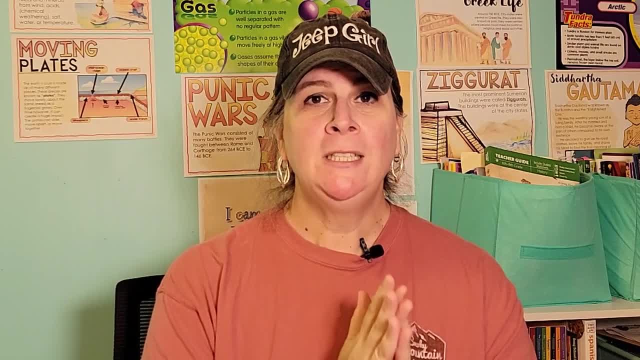 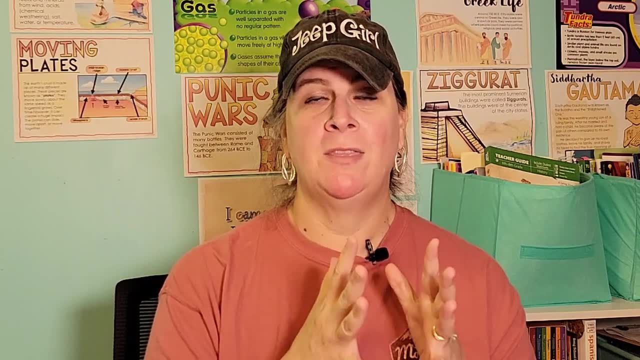 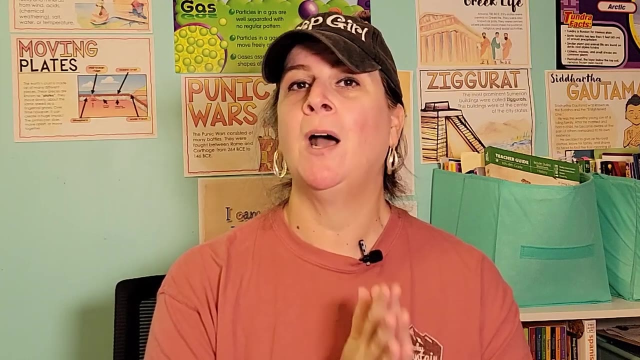 math. This is something that I feel really strongly about, And so if you have a student who is thriving in the math curriculum that you have chosen for them and they it is working well, then I recommend that you stick with it, if possible. Now, the reason, again, that we did not stick with what we were doing is because it wasn't. 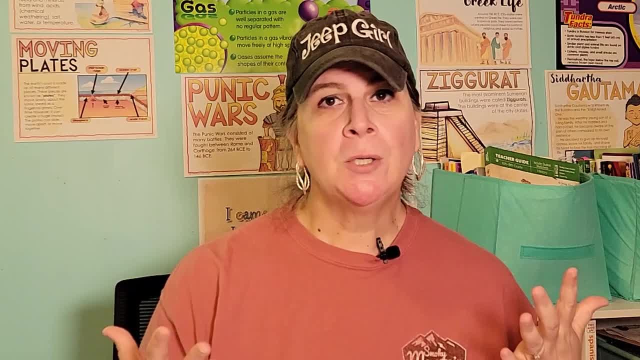 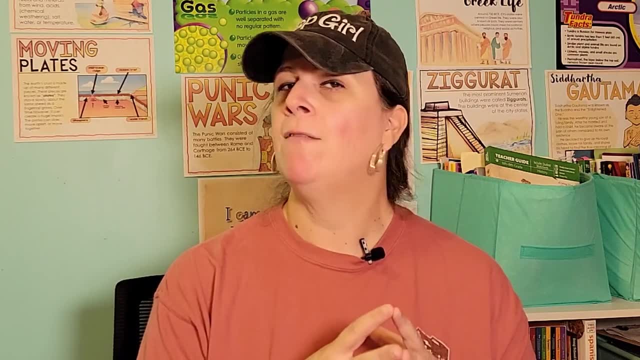 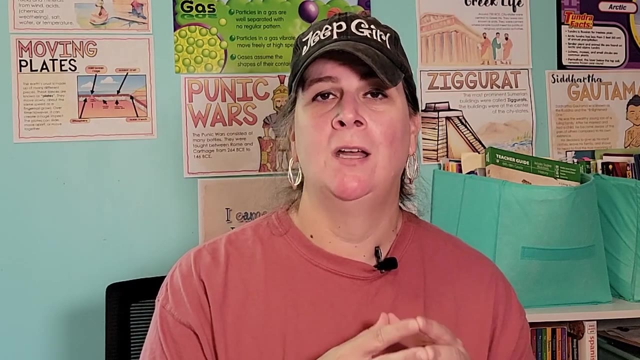 it was no longer going to work. Singapore Dimensions 7 was no longer going to work for us. We were going to have to switch at the end of eighth grade. Anyway, because Singapore Dimensions does not have math past eighth grade, The price tag is definitely something I want to note in discussing these math curricula. 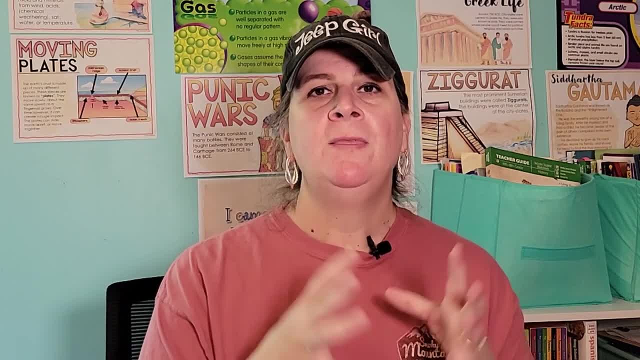 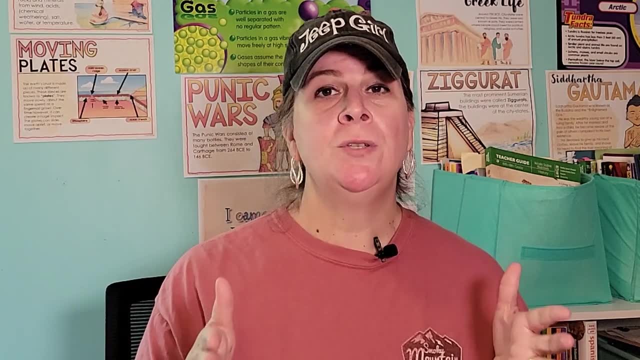 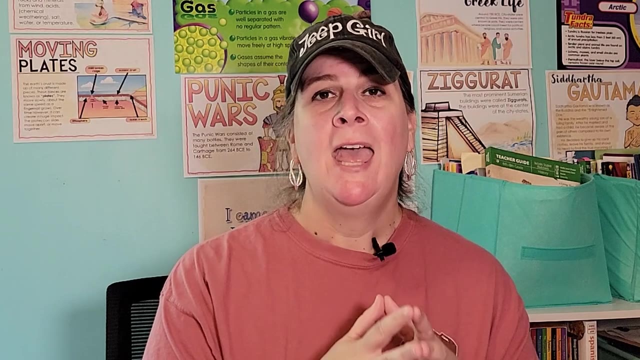 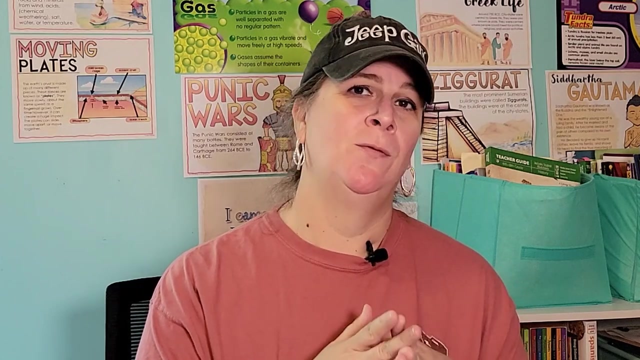 In general, they are between $100 and $300 a year. This is just for either the textbooks up to the pre-recorded classes. If you choose to do live classes with your student, then that price definitely increases, And so I want to note that the price for live classes is much greater than the price for those pre-recorded. 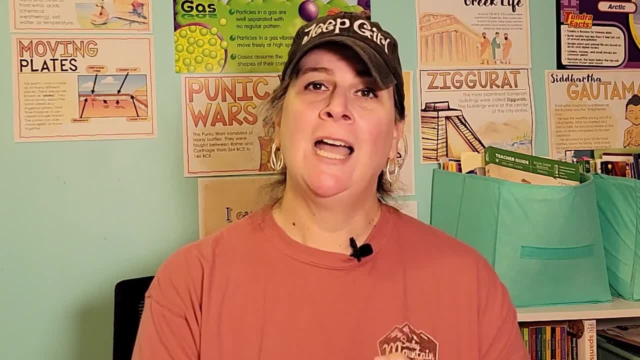 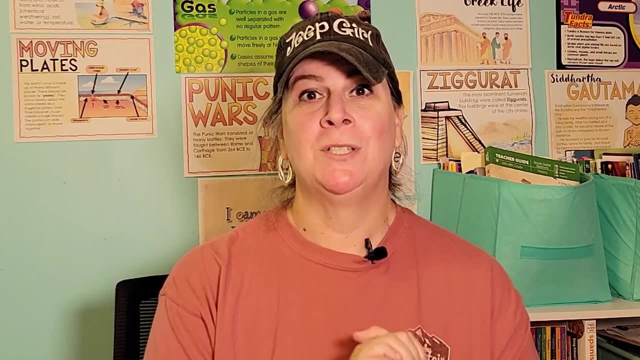 classes. So let's get started. The first one that I looked at was Denison Algebra. I am so impressed with Denison Algebra. I was able to talk to Mr Denison when I was at the Teach Them Diligently conference. 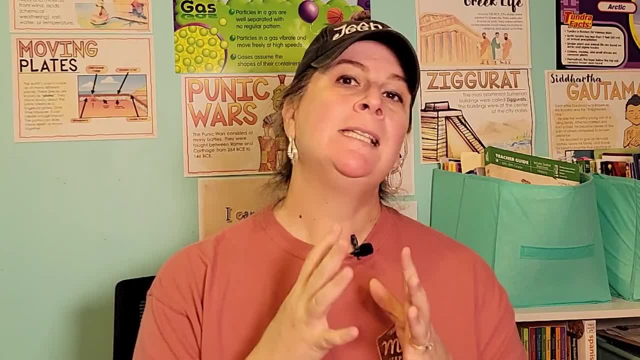 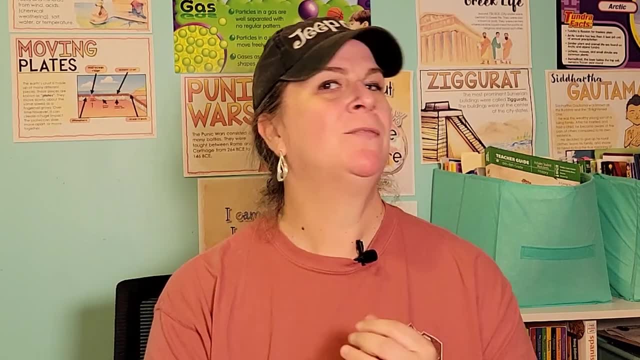 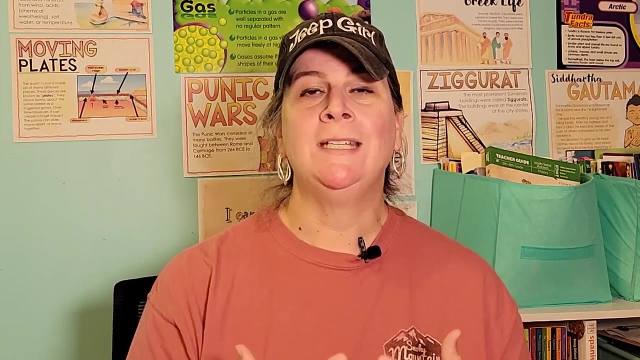 And he is absolutely amazing. He has a heart for students to learn math. I also appreciate him because he was very honest with me. When I talked to him about my daughter's strengths and her weaknesses and what I wanted, he honestly informed me that Denison Algebra was not for us. 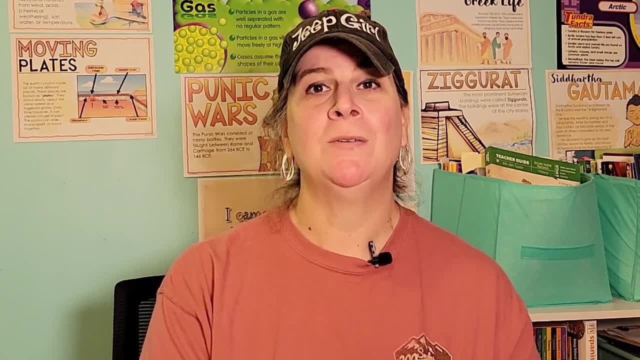 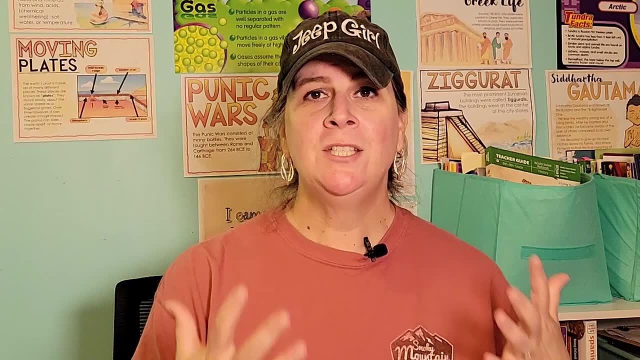 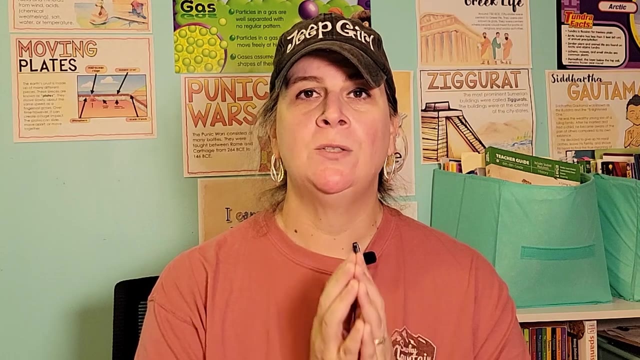 Now Denison Algebra does have the textbook that I wanted. It has the videos that I wanted. He is adding classes, So it is going to be a curriculum that will grow and she would be able to continue it through high school. However, Denison Algebra is really focused towards the student that doesn't like math. 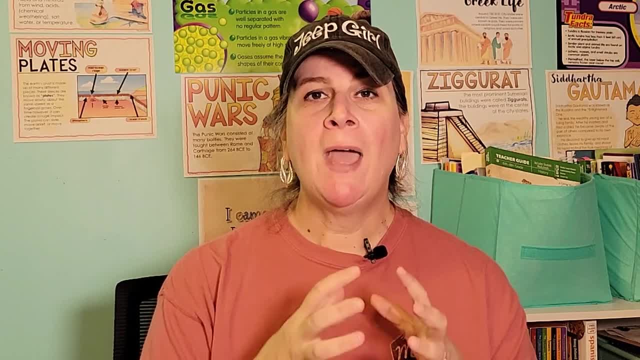 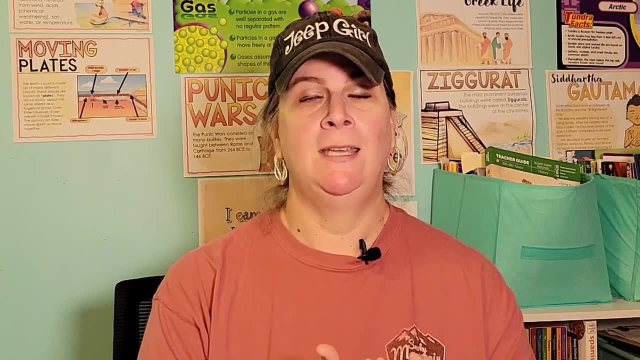 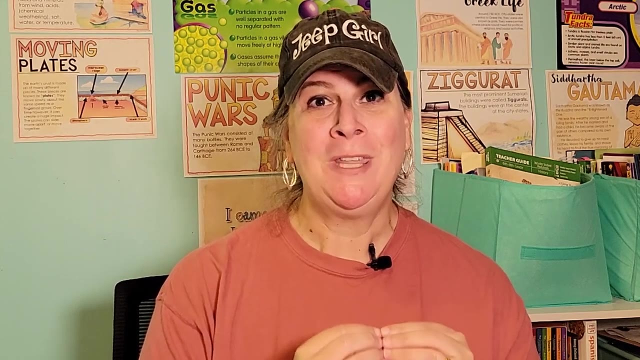 The student that struggles some with math. So if you have a student who doesn't like math or struggles, I highly recommend that you reach out to Mr Denison and Denison Algebra and see if he thinks that this is correct for you. He will be honest with you. 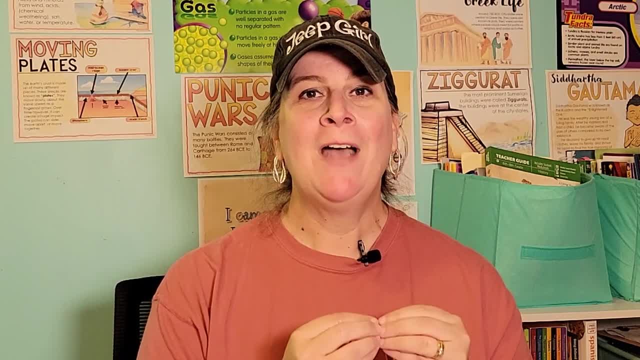 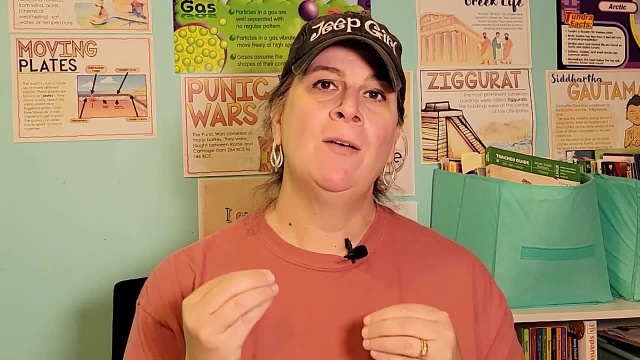 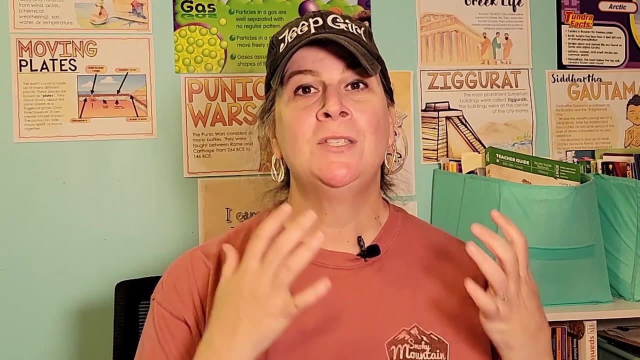 And so definitely reach out to him. I have learned through talking to other people. I have learned through talking to other people. He has been honest with them too. He has been honest when he thinks that his program will work with their students, and he has been honest when he thinks that their program won't work with their students. 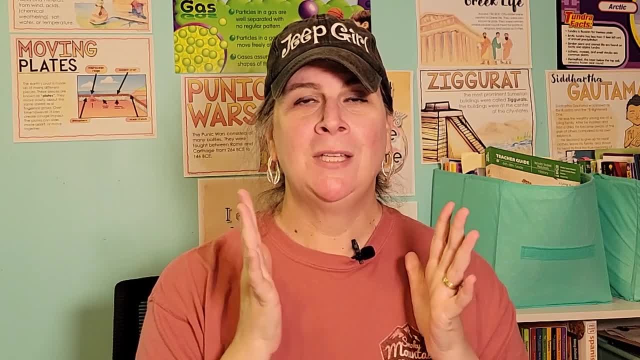 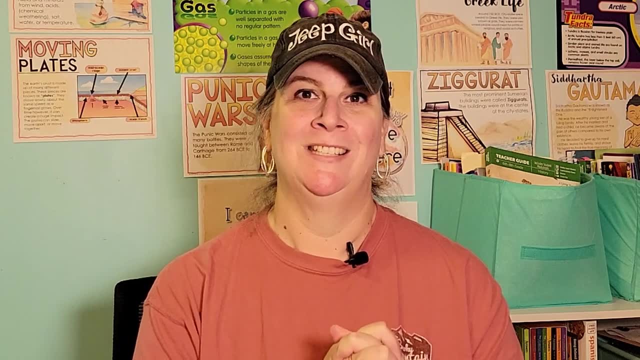 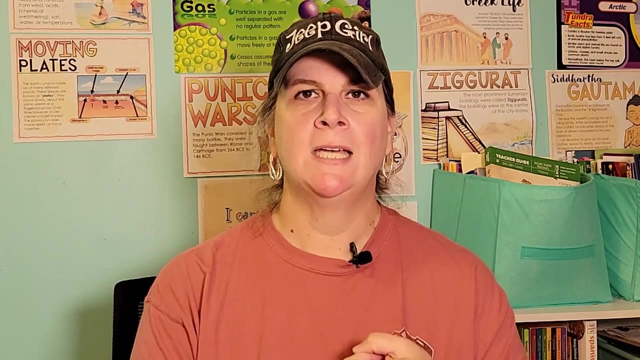 So definitely check out Denison Algebra. I am extremely impressed with the program, with Mr Denison and with his love for students. The second program that I looked into is Shorman Math. Shorman Math does have the video components. It doesn't really have a textbook. 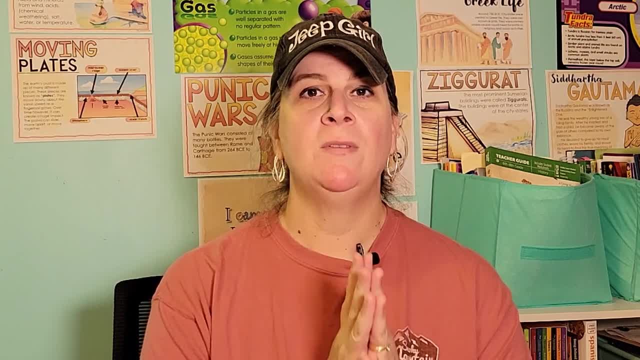 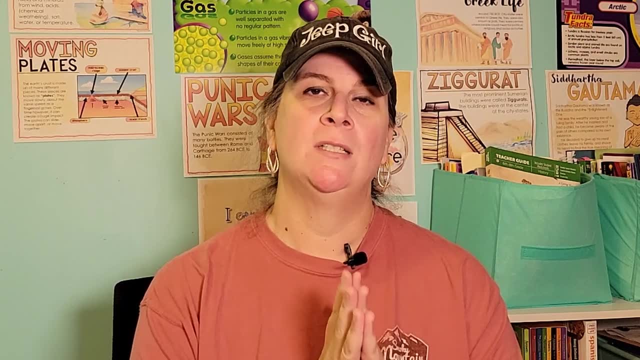 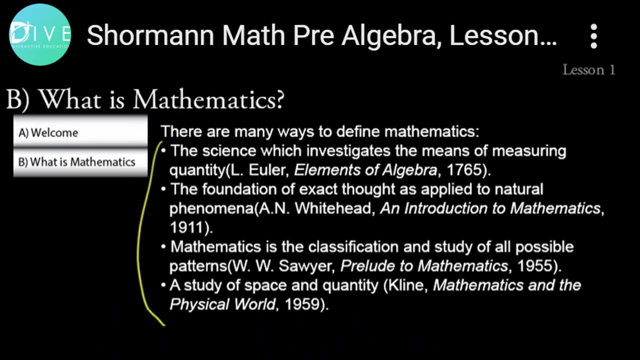 It is more of printing off sheets when you need to. There is quite a bit of text on the screen, And this was something that I really thought was not going to be good for my daughter if she was learning directly off of a screen without that textbook in hand. 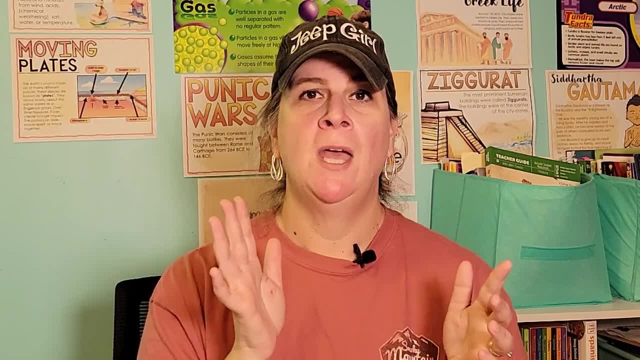 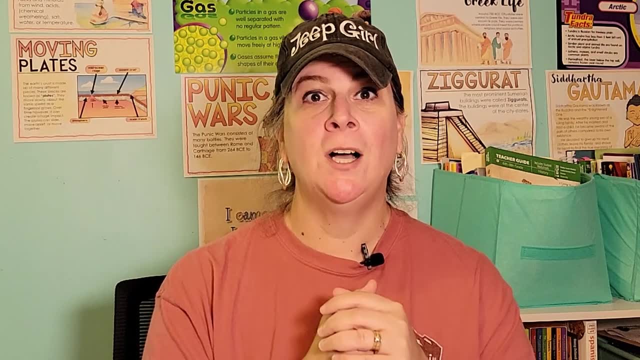 Now, Shorman Math is designed for students who are going to college. So if you have a student who is going to take the PSAT, the SAT, the ACT, Shorman Math is designed for this. Also, if you are going to college, you can use the PSAT. 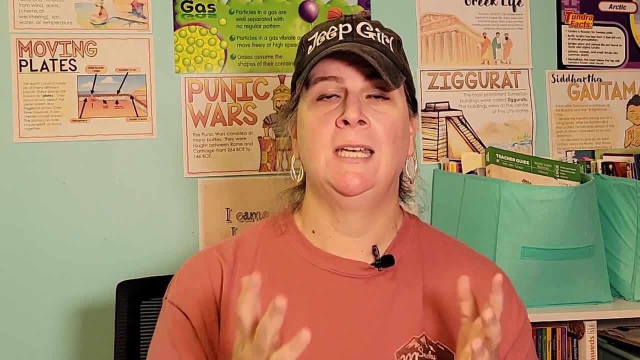 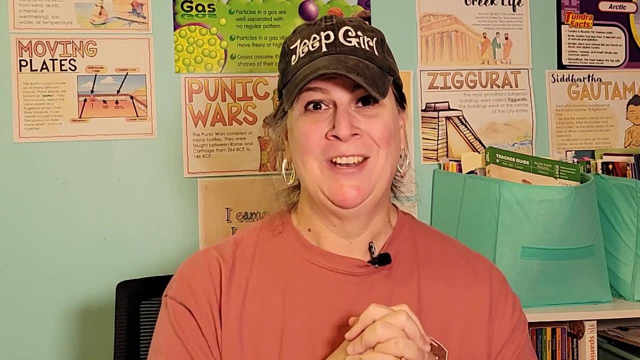 So if you take Algebra 1 and Algebra 2, then you can get a geometry credit as well. So that's three credits for the two classes, which is, you know, awesome. But Shorman Math just really did not seem like something that would work for my daughter. 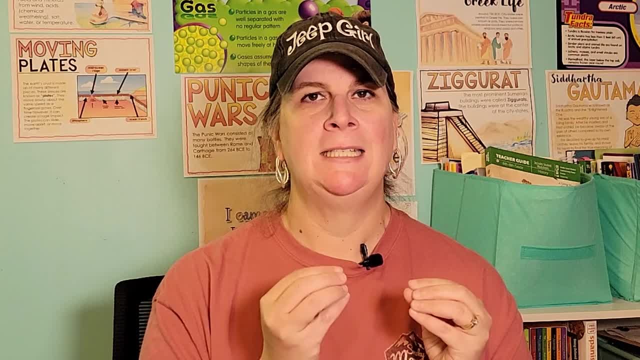 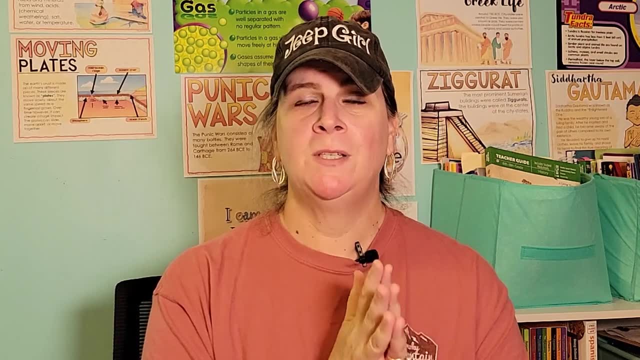 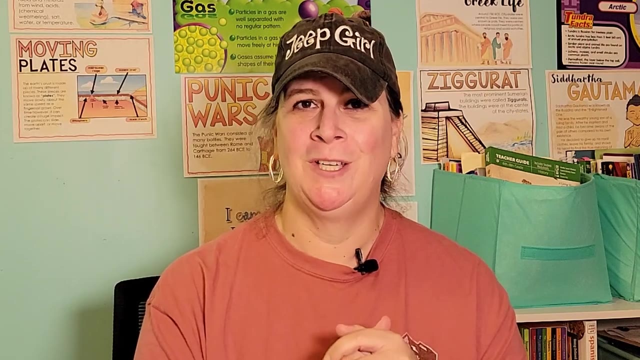 based on her learning style. I need that textbook right now, But if you have a student who has a Saxon Math background, loves Saxon Math and needs to switch for whatever reason, Then I would recommend looking at the textbook, Looking into Shorman Math, because it may just be the perfect fit for you. 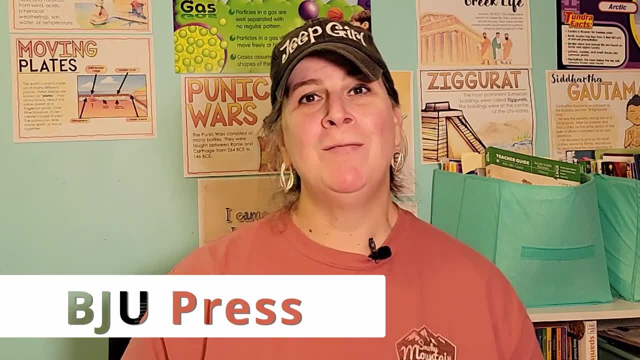 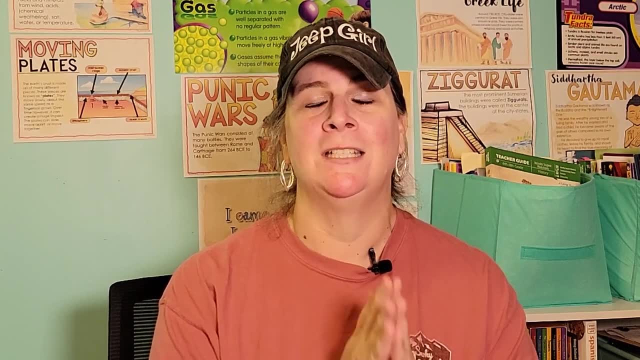 BJU Math is the third math that I looked into And I have to say I was impressed with BJU Math. It definitely is one that I kept going back to and looking at. BJU Math is in the process of redoing their pre-algebra program. 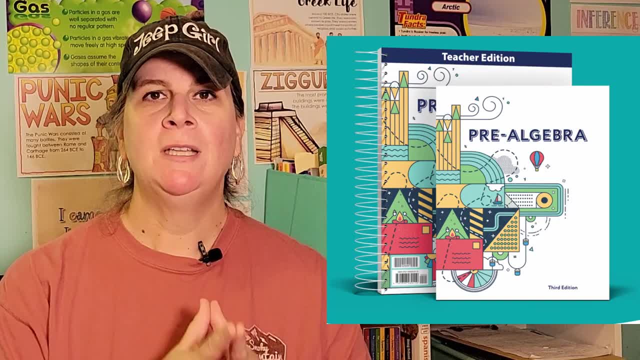 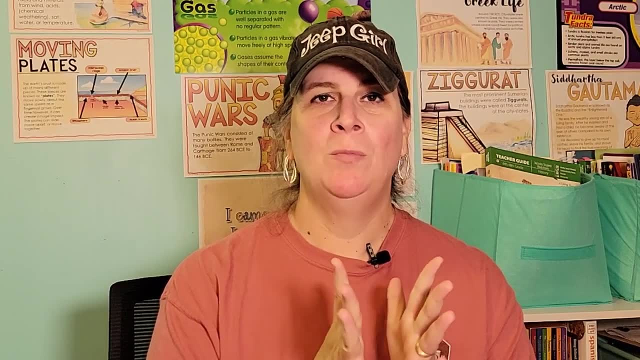 Pre-algebra is considered an eighth grade math for BJU And they will be releasing an updated pre-algebra curriculum at the end of June 2023.. BJU Math has some wonderful components. You have the student text, the teacher's manual. 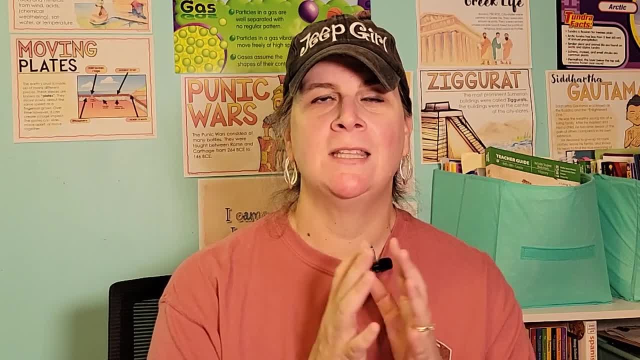 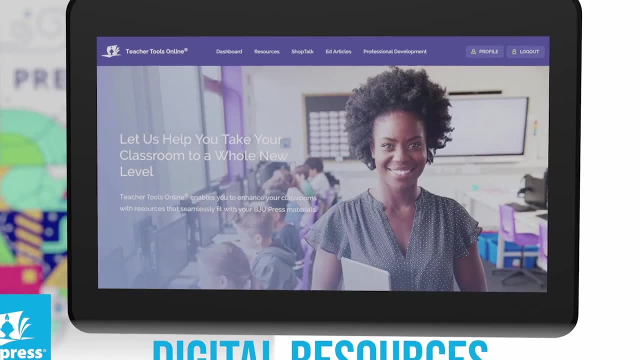 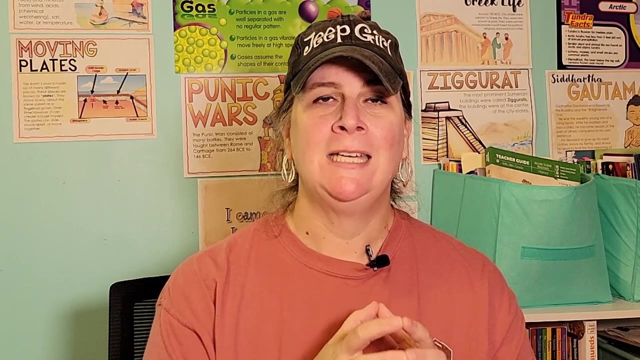 You also have tests and quizzes. There's activities. There's so much included in BJU Math. Additionally, BJU has a video component that you can utilize with the BJU Math, And it is something that I really liked. Now, One of the things about BJU Math: 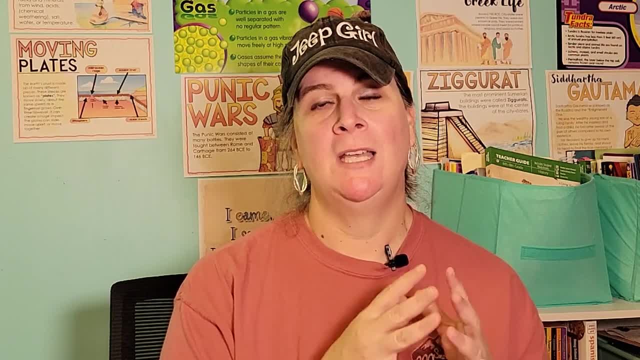 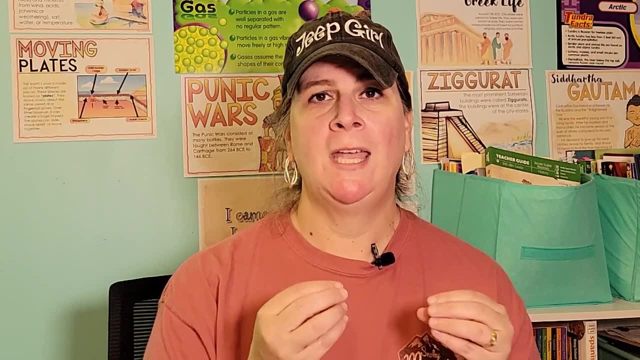 At least the article, The article, The older versions, The ones that I was able to look at when I was at the Teach Them Diligently conference. It is much more of a traditional math. There are problems on the page, You memorize how to do them and you just keep on going. 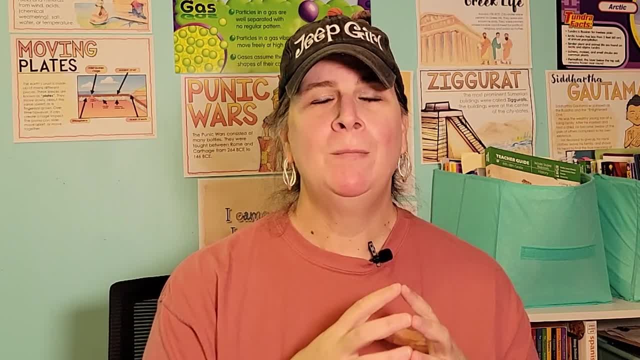 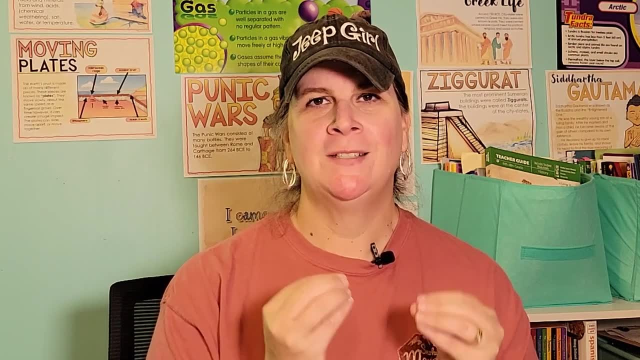 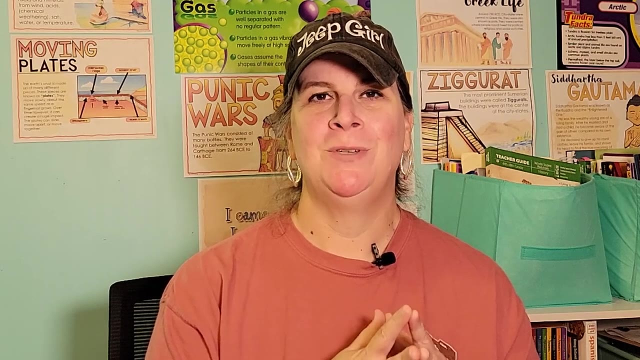 It is a spiral approach, but I wanted more from math if possible. I wanted that. why I wanted for my daughter to understand the why of things, versus just memorizing How to do the problems and then being able to move on. I really wanted to solidify a lot of the why. 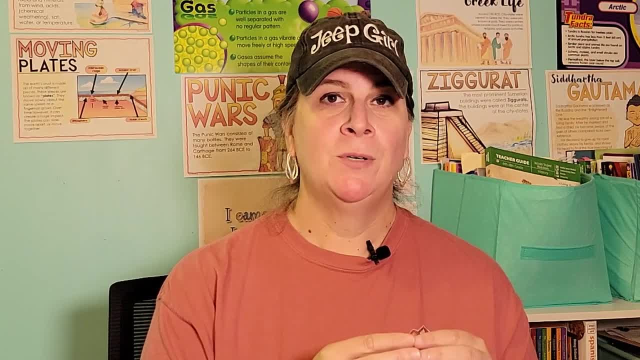 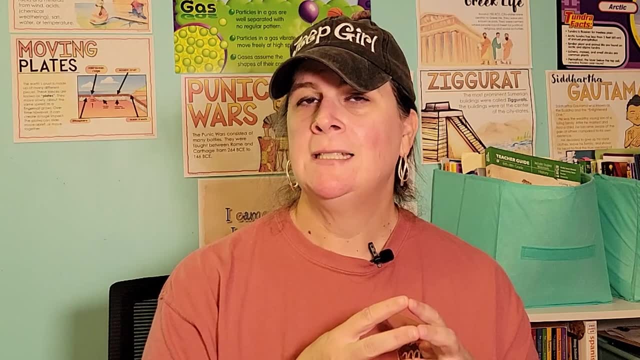 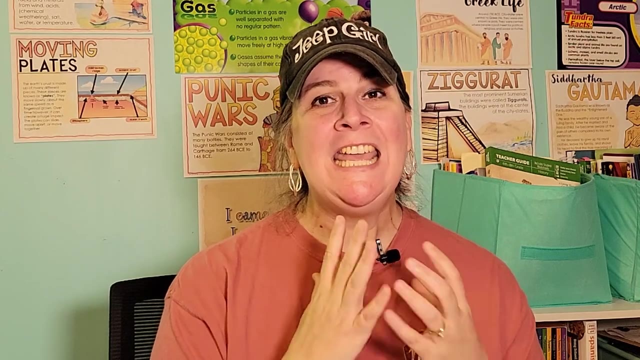 Which is why we originally switched over to Singapore Dimensions- is because they drew focus on that. why? So that is really the biggest reason that I stepped away from BJU- is because of the why. Now I will just say: If what we are doing does not work out, 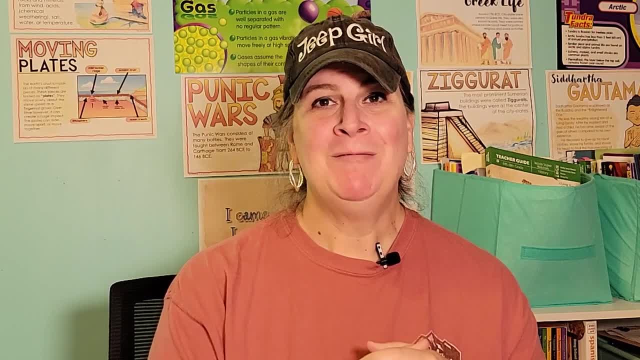 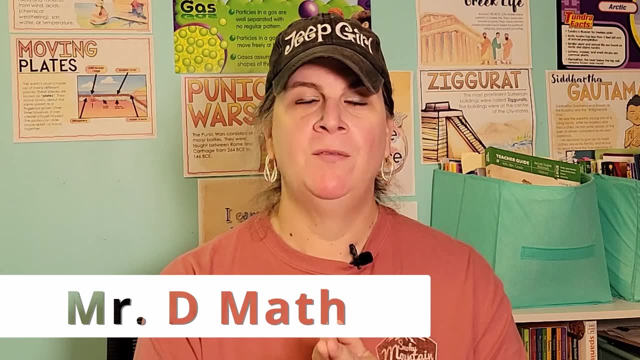 I am going to revisit BJU because I was impressed with BJU Math. Next is Mr D Math, So Mr D Math does have either a live or a self-paced option. Again, this is one where there is not the textbook. 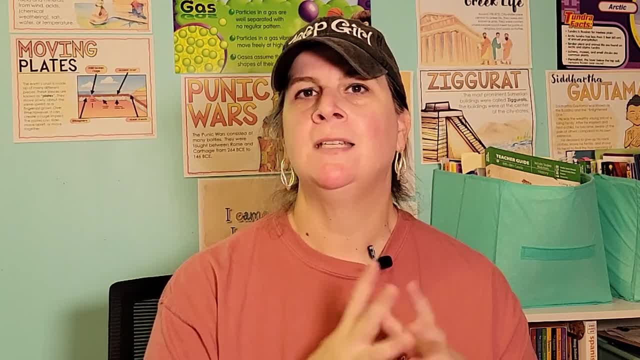 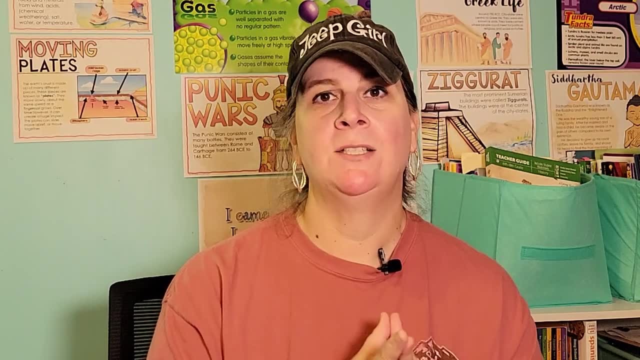 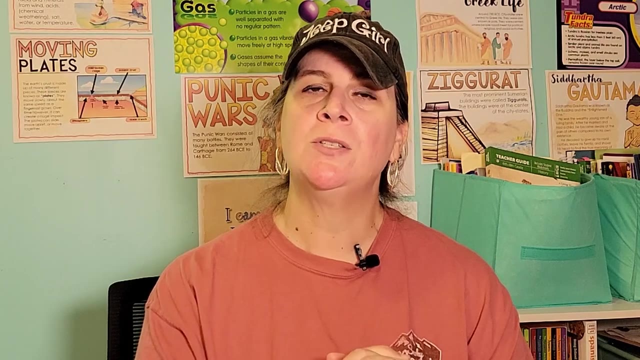 I need that textbook and that was really the main reason that I eliminated Mr D Math. They do have pre-algebra up through calculus. There is also the opportunity to have access to a live teacher three times a week if you need it. Mr D Math did have a lot of really good components to it. 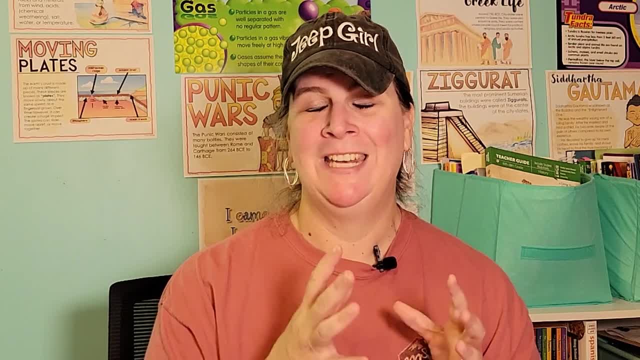 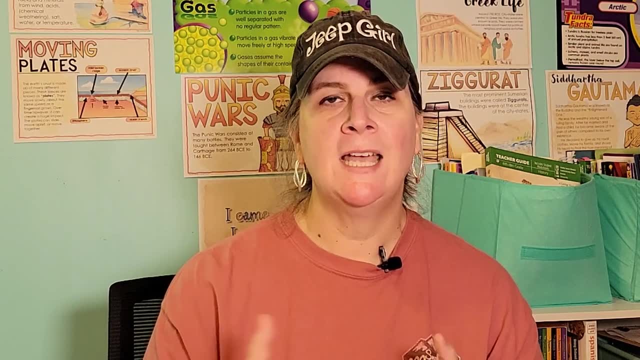 It really is just that textbook that I wanted in it for math not to be totally online. If you do choose the self-paced option, there is an 18 month access. I highly recommend that you look at the live versus self-paced document that Mr D Math. 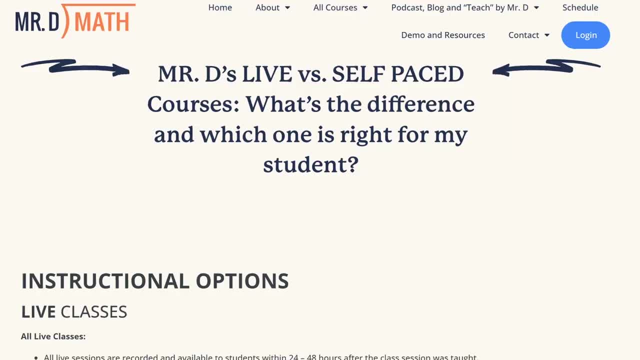 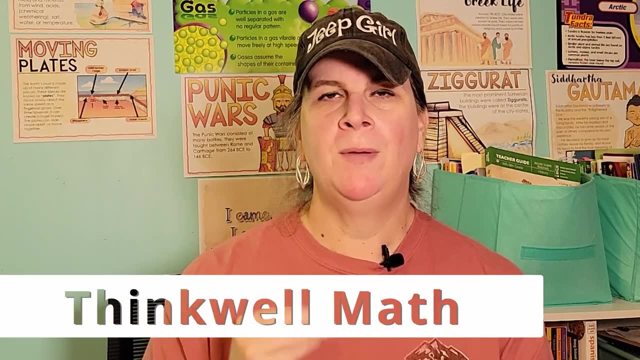 offers on their website. It is a wonderful comparison of these two approaches within Mr D Math, So take a look at that if you are considering Mr D Math. I did review Think Well Math. Based on what I have heard about it, it does seem to be a rather advanced math program. 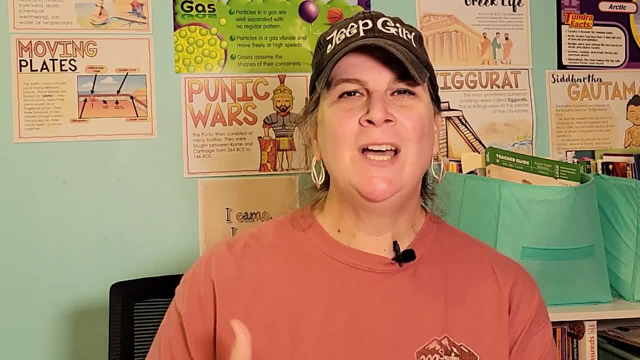 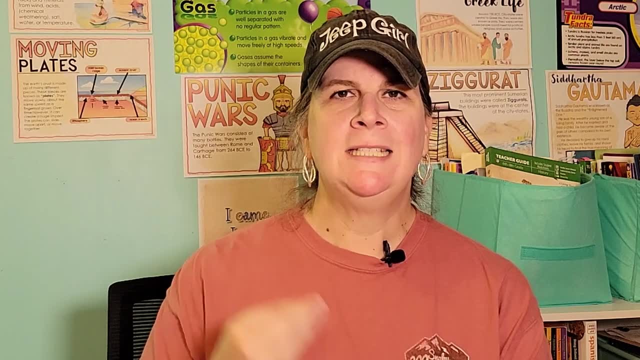 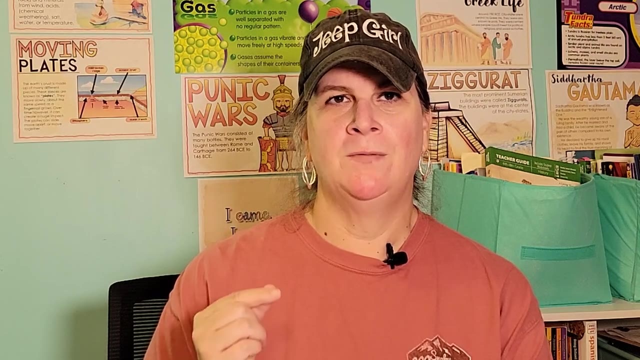 It does have pre-algebra up through calculus. There are downloadable notes and worksheets, and then you have the video instruction. One of the reasons that I didn't dive anymore into Think Well Math is because of just the video instructions, versus me being able to have a teacher's manual. 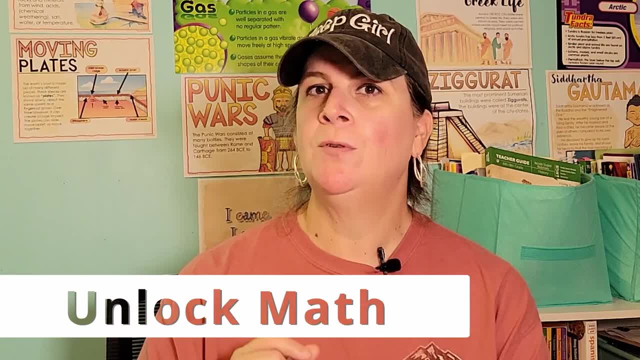 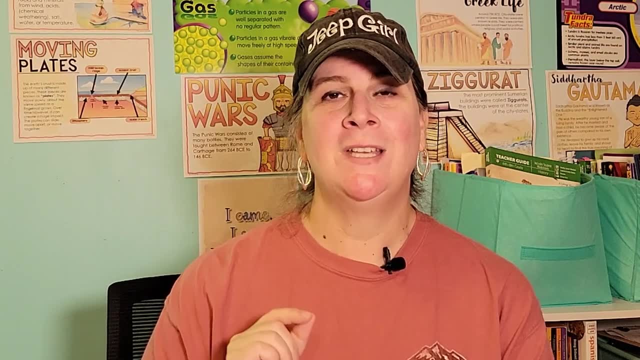 The next one I looked into was Unlock Math. Unlock Math does have a 14 day free, So if you are interested in it, please make sure that you check out their free trial. One of the videos that I was most impressed with is when the teacher was talking about. 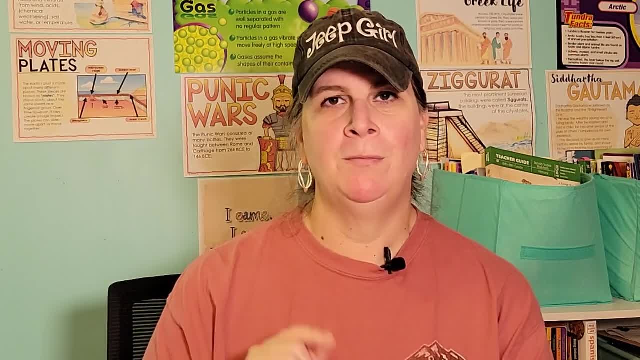 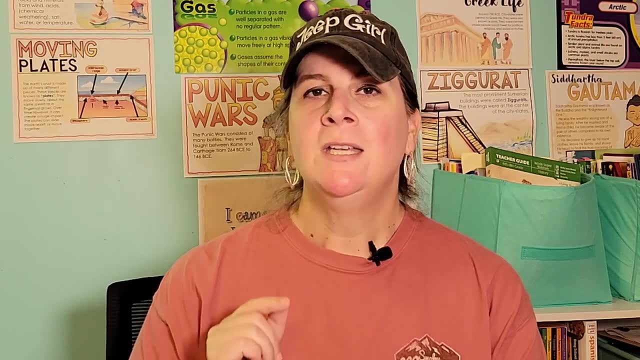 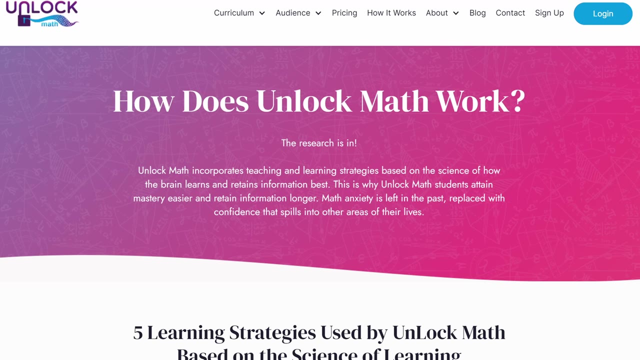 finding the relationship between circumference and diameter. I really liked that video and it was actually one of the ones that sold me the most on Unlock Math. Now there are short video lessons and then you do your individual lessons. There are testing quizzes that you also can do. 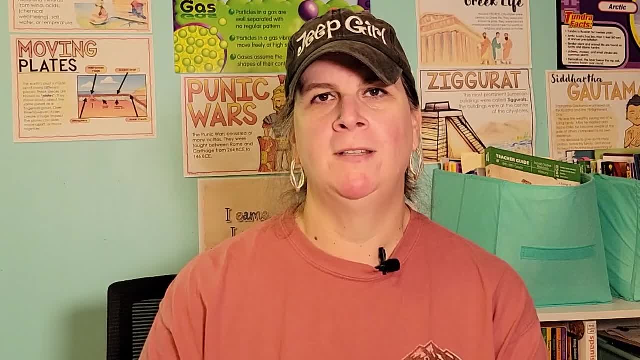 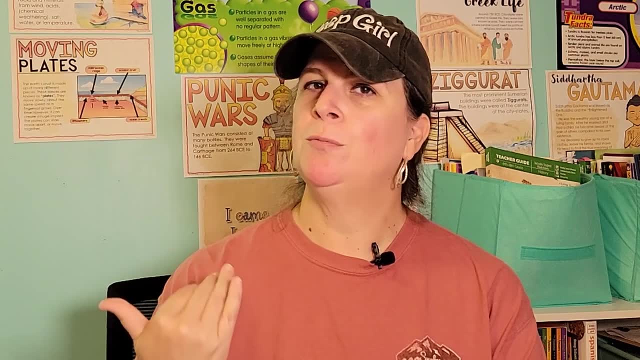 There is a video lesson that you can do. You can also take, but this, again, is all online. There is not a textbook, which is something that I prefer Also Unlock. Math goes through pre-calculus at this time and not through calculus- Again, something that I was looking for. 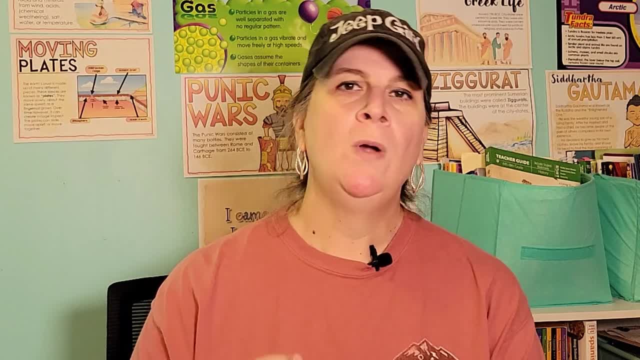 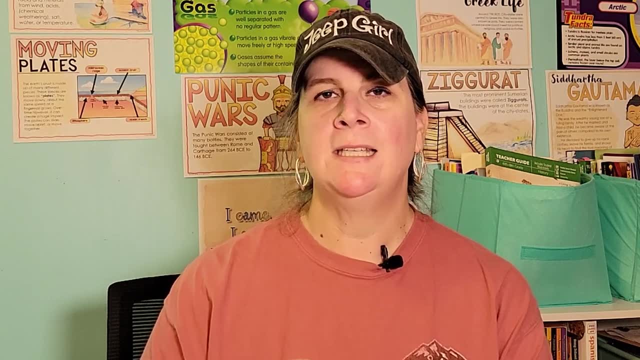 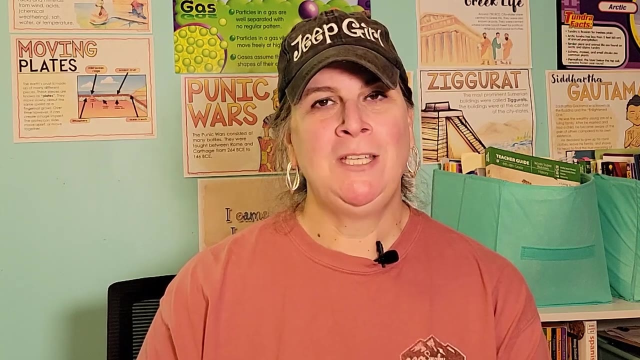 But I have to say the lessons that we have done within Unlock Math have been amazing. I love the way that the teacher teaches these lessons. It is great for the supplement that I was looking for If we needed it, And that leads me to the art of problem solving. 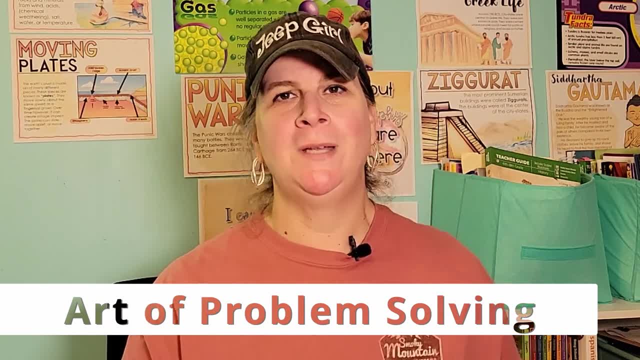 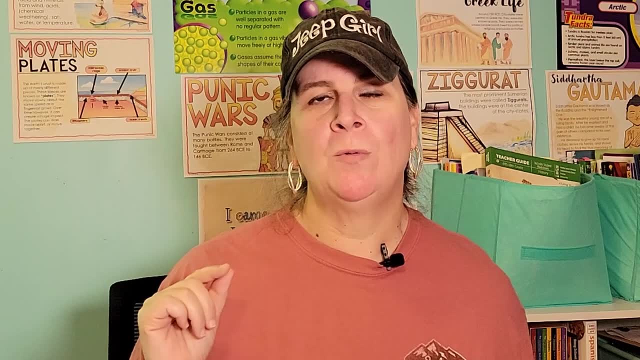 Now, if you saw my seventh grade curriculum picks, you know that we did choose the art of problem solving. This is what we will be using. I am putting it together with Unlock Math and I will talk about that in another video. But the art of problem solving. 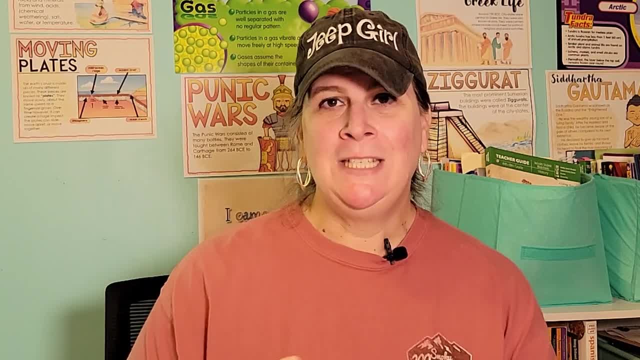 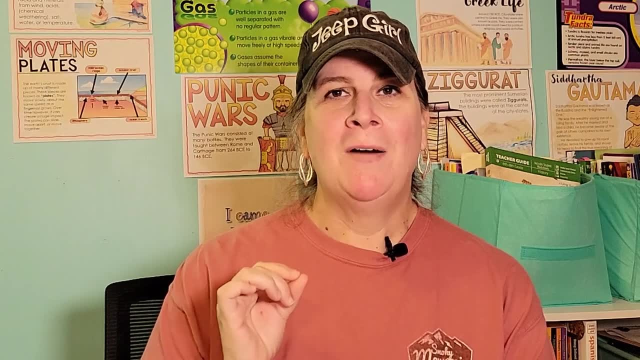 Here are the reasons that I chose it. Number one: it teaches you how to think. Art of problem solving is something that you can do. You don't have to be a math teacher that you have to think about now. I'm interested to see how this works with my 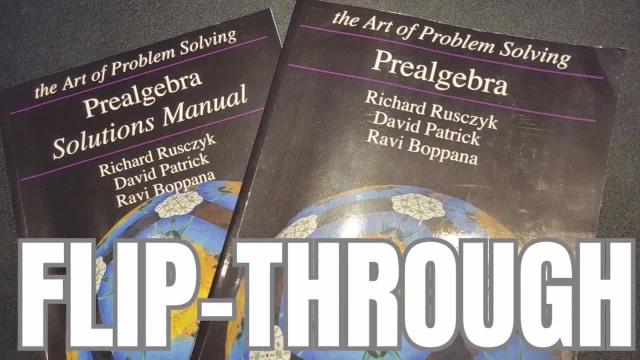 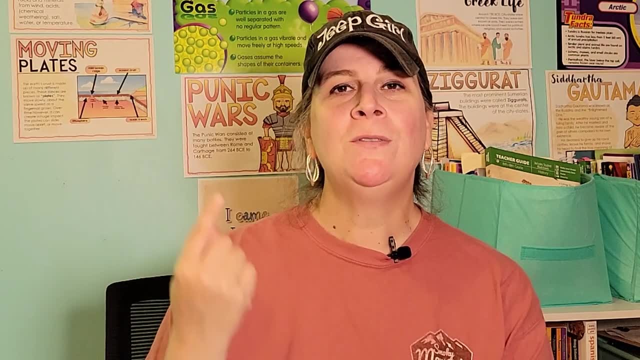 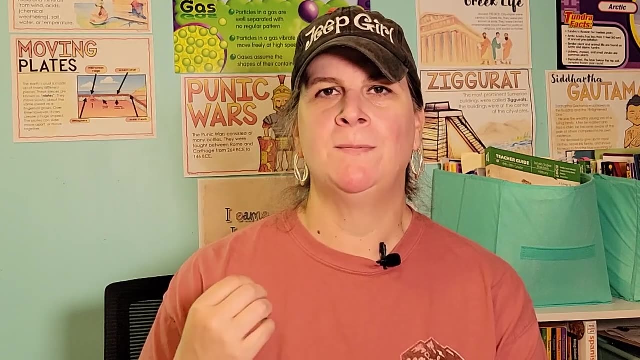 daughter, because at the beginning of the lessons you may be given those questions and they ask you to solve them, but you haven't been taught anything yet. so they want you to think about it and to reason through those questions, and I like that because you're not always going to have a specific formula for how to do life. 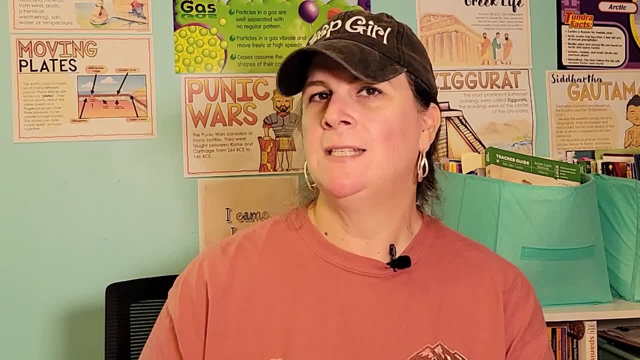 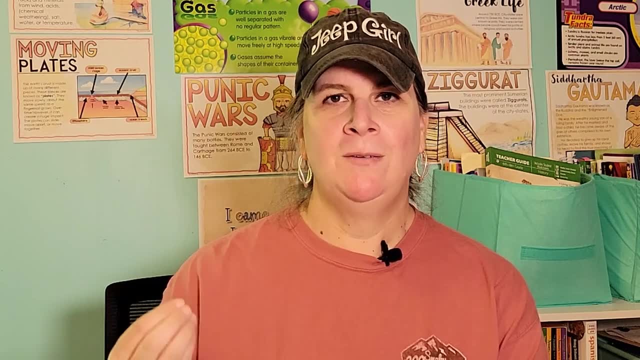 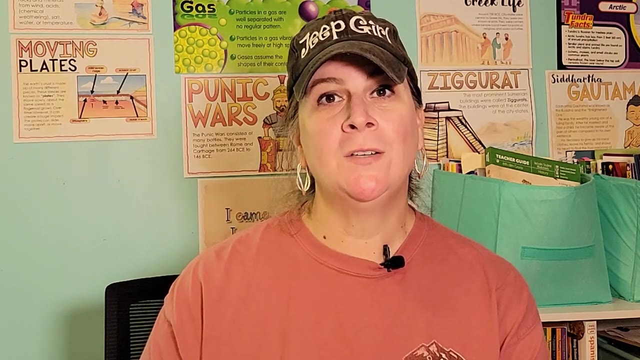 and just having that critical thinking component is something that I'm really excited about. and then they go through and they teach you about the concept and you have your question, the additional questions at that point. also, art of problem-solving has wonderful videos that are free, that you can utilize to go. 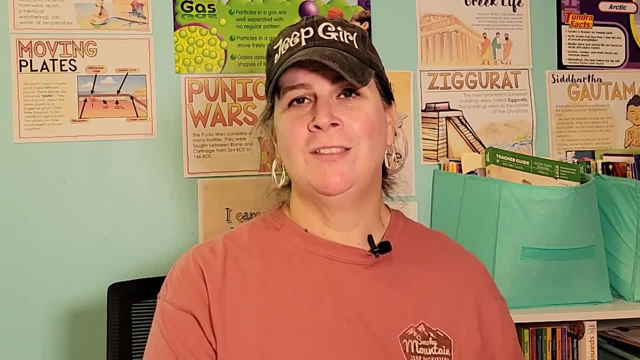 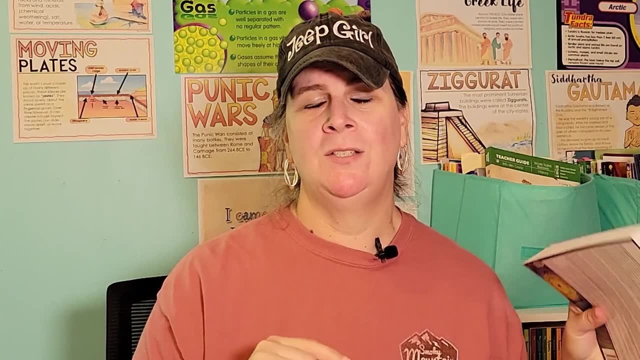 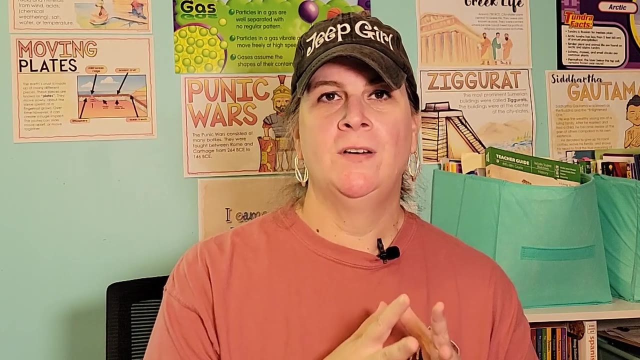 with the lessons. additionally, as you saw, there is a textbook, so I do like the fact that there is a test textbook. if you buy the textbook, then you should also purchase the answer book. if you would like online classes, they offer that as well. each one of the math: